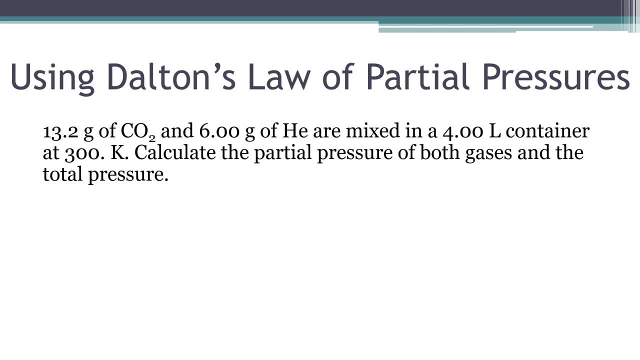 dioxide and 6.00 grams of helium are mixed in a 4.00 liter container at 300 kelvin. Calculate the partial pressure of both gases and the total pressure. Because we have a mixture of gases, we'll use the ideal gas law to find the partial pressures for each gas, Then use Dalton's. 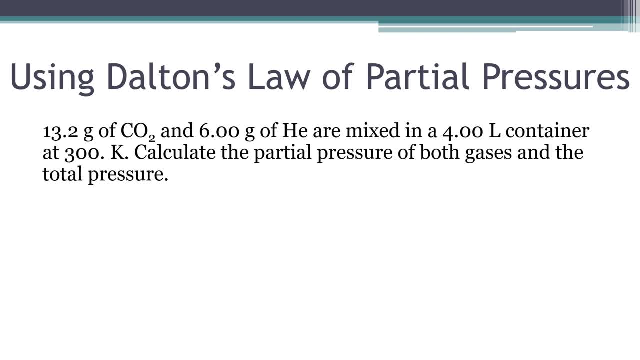 law of partial pressures to find the total pressure by simply summing the partial pressures. First I'll convert the masses to moles using the molar mass for each gas. Next I can use the ideal gas law to find the partial pressures. Note the only term. 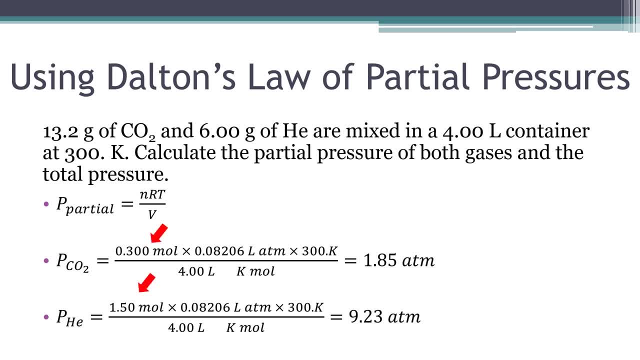 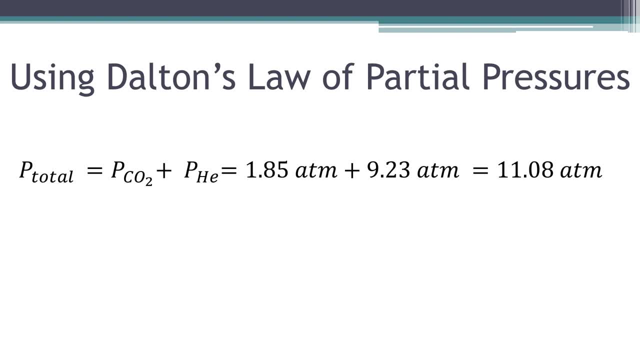 that's different is the moles of each gas. Now I can sum the partial pressures to find the total pressure. The total pressure is 11.05 grams of hydrogen. The total pressure is 11.08 atmospheres. But note, the total pressure could also. 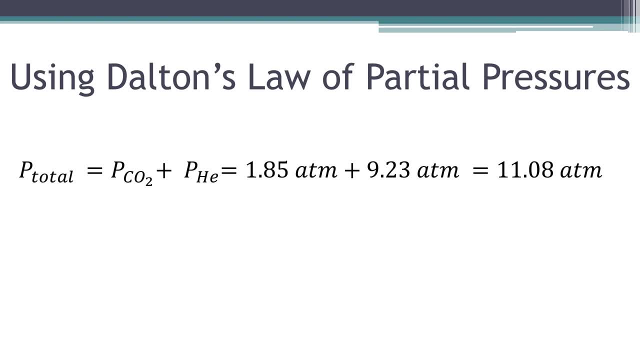 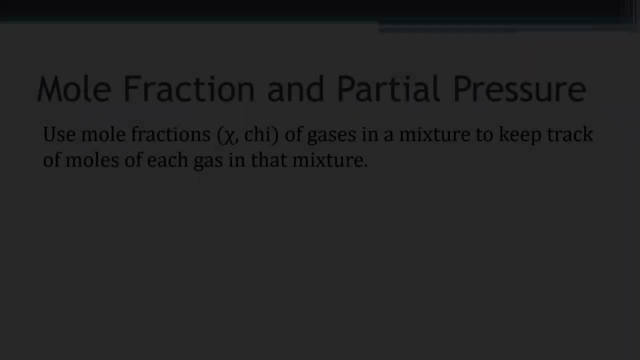 have been solved by summing the moles of the ideal gases. I could have used the total moles and reached the same total pressure to three significant figures. We can use mole fractions of gases in a mixture to keep track of the moles of. 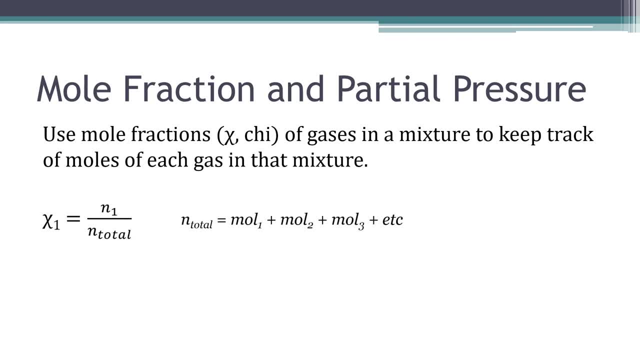 each gas in that mixture. The mole fraction is denoted by the Greek letter chi. In this example, the mole fraction of gas 1 is the moles of gas 1 divided by the total moles in the mixture. And why would we need to know the mole fraction? The mole fraction can. 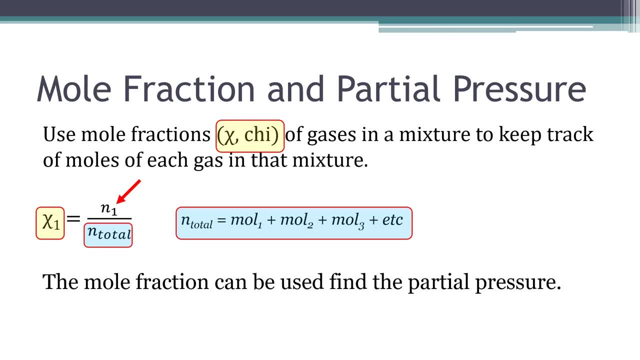 be used to find the partial pressure of a gas in a mixture. Here, the partial pressure of a gas is the mole fraction times the total pressure of a gas, The pressure which is known as the mole fraction times the power of a gas. 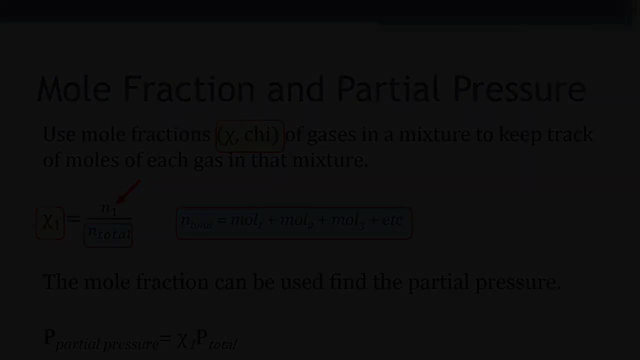 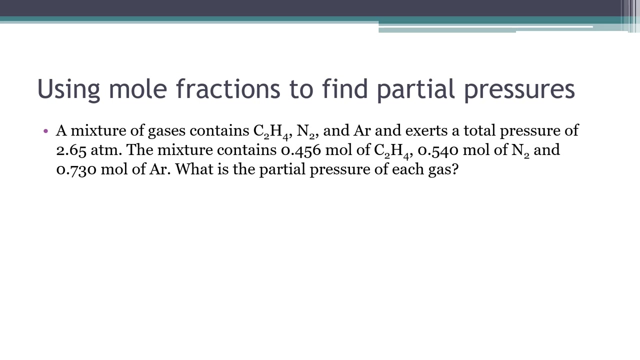 This is the pressure of the mixture. Here's an example of using mole fractions to find partial pressures. A mixture of gases contains ethene, nitrogen and argon gases and exerts a total pressure of 2.65 atmospheres. The mixture contains 0.456 moles of ethene, 0.540 moles of nitrogen and 0.730.